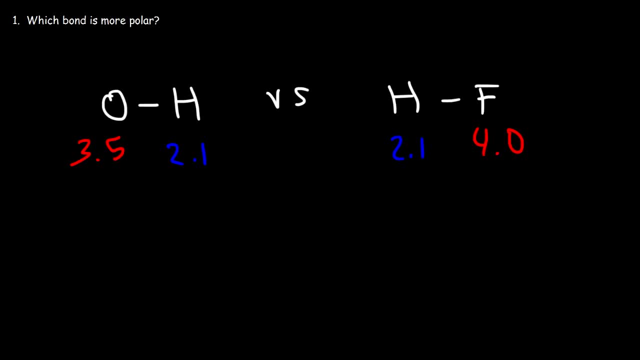 Fluorine is the most electronegative element that we know on a periodic table. Now the En difference for the OH bond is 1.4 and the En difference for the HF bond that's 4 minus 2.1, so that's 1.9.. 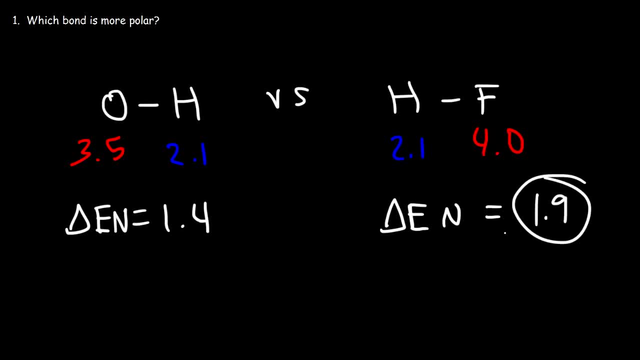 So because this has a higher electronegativity difference, we could say that the HF bond is more polar. Now, both of these types of bonds, they represent a special class of bonding, particularly hydrogen bonds. Whenever you see hydrogen attached to nitrogen oxygen or fluorine, you have a special case of hydrogen bonding. 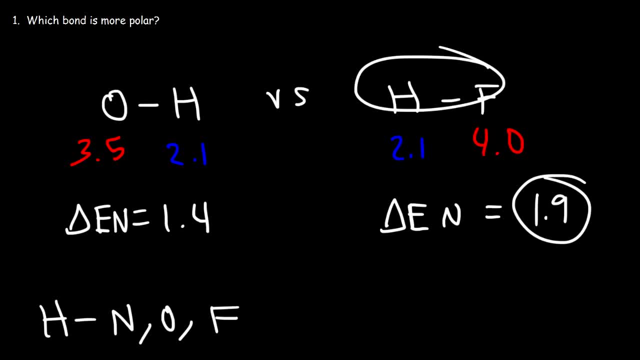 But this is going to be the most polar covalent bond that we have here. Now we need to indicate the direction of polarity. So oxygen is more electronegative than hydrogen, so it's going to have the partial negative charge. Hydrogen is going to bear the partial positive charge. 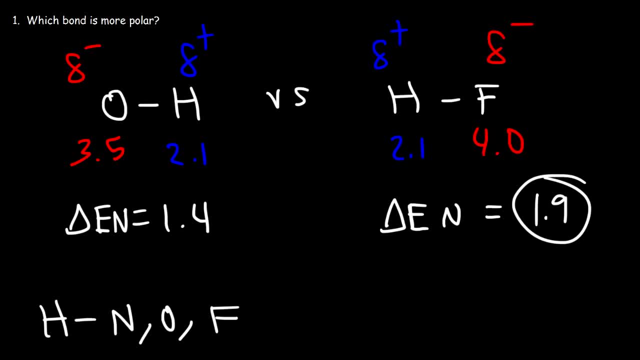 And fluorine is more electronegative than hydrogen. To draw the dipole moment, you need to point the arrow towards the more electronegative element. So you can do it like that. Now, what if you don't know the electronegativity values? 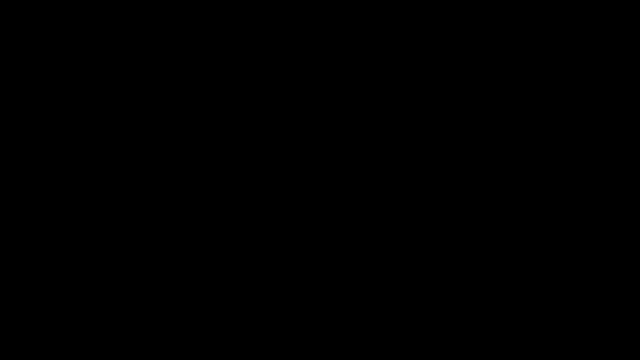 Let's say you're taking a test And you just don't remember what the numbers are. What can you do in a situation like that? So here's an example that will illustrate what you can do in such a scenario. So let's consider the carbon-nitrogen bond and the carbon-oxygen bond. 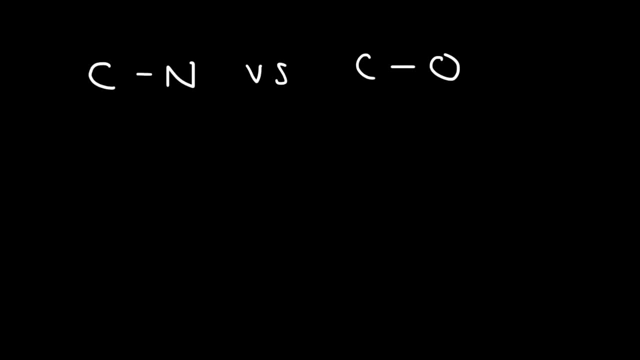 So which one would you say is more polar? What you need to do is locate the periodic table. On the periodic table, you'll have hydrogen, boron, carbon nitrogen oxygen and fluorine laid out like that. So notice that we have the same element, carbon. 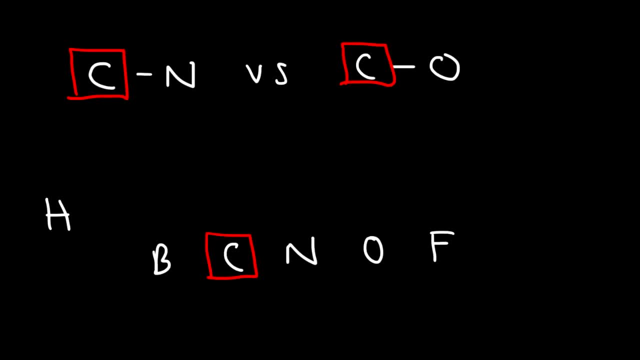 So that's our reference element. So we're comparing carbon and nitrogen to carbon and oxygen. So notice that carbon and oxygen are further apart than carbon and nitrogen provided that they're in the same row, And so whenever you have two elements that are further away from each other in the same row, 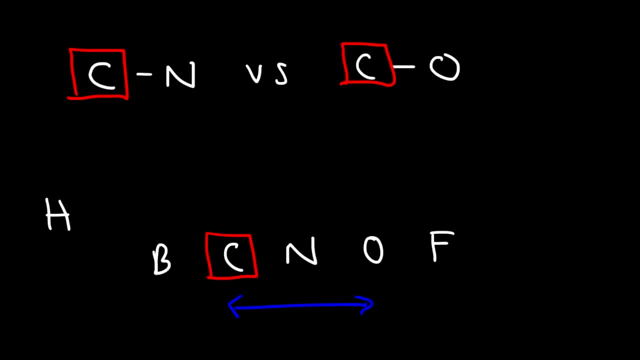 they're going to have a greater difference in electronegativity, Because electronegativity increases towards fluorine. It increases as you go to the right and as you go up across the periodic table, And so the electronegativity difference between carbon and oxygen is going to be greater than carbon and nitrogen. 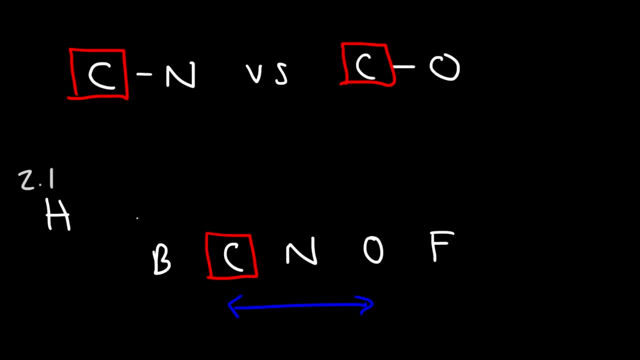 Here are the numbers: Hydrogen is 2.1, boron is 2.0, carbon is 2.5, N is 3.0, O is 3.5, F is 4.0.. And so 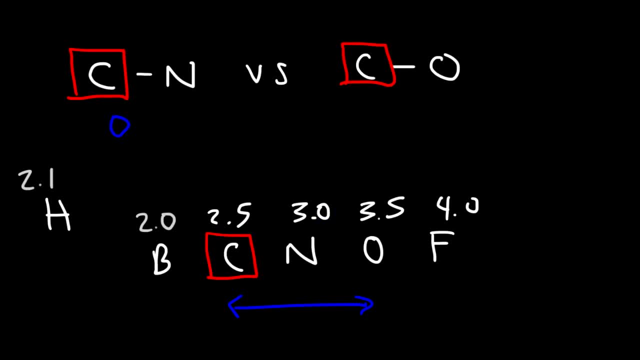 The difference between these two numbers is only 0.5.. But the difference between these two numbers is 1.0.. So whenever you have two elements that are far apart from each other, typically they will represent a more polar bond than two elements that are closer to each other in the periodic table. 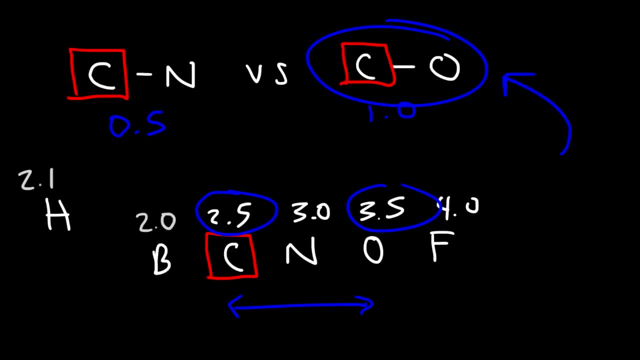 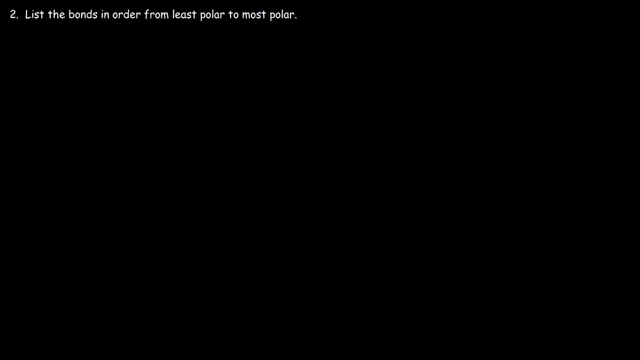 So CO is the most polar out of the two that are listed here. Here's another problem for you List the bonds in order from least polar to most polar, And so let's say we have the carbon-bromine bond, the carbon-iodine bond, the carbon-chlorine bond and the carbon-fluorine bond. 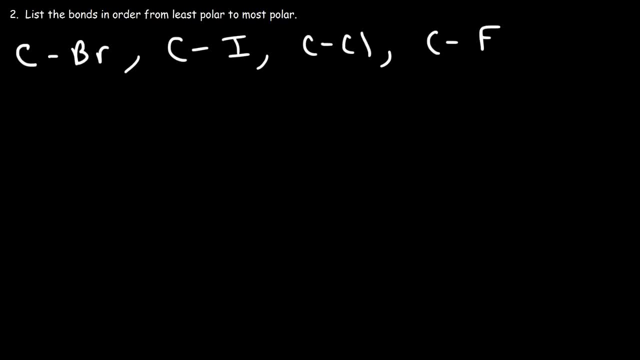 So go ahead and try this. Now we know the electronegativity of carbon: It's 2.5.. But what about the halogens? So let's see if we can do this without using the numbers. But then we'll confirm it with the numbers. 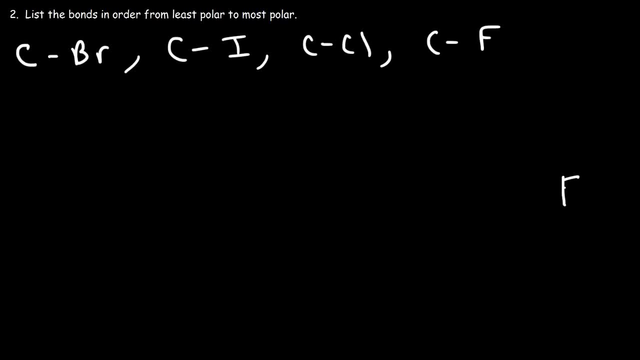 On the periodic table. the halogens are listed in this order. Now you need to keep in mind that electronegativity increases as you go up, And so fluorine is the most electronegative halogen in this group Now, given that carbon has the same electronegativity value. 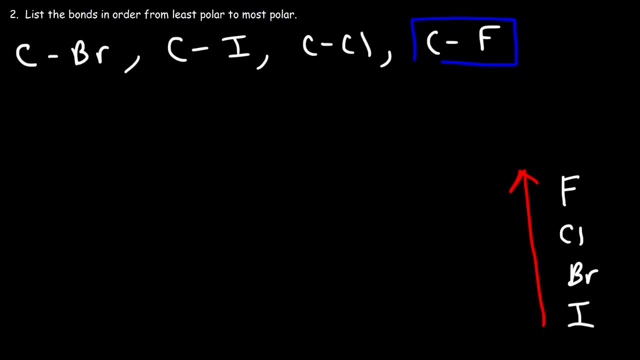 we could say that CF is going to be the most polar, since it has the most electronegative element in it, And then it's going to go in order. So we want to rank it from least polar to most polar. So iodine has the lowest electronegativity value out of the four halogens. 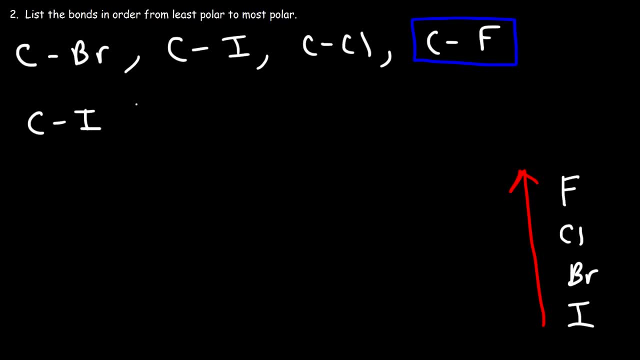 So we could say that it's going to be the least polar, So it's going to be Ci, and then that's less polar than CBr, which is less polar than CCl, and that's less polar than CF. So once you identify the most polar group, 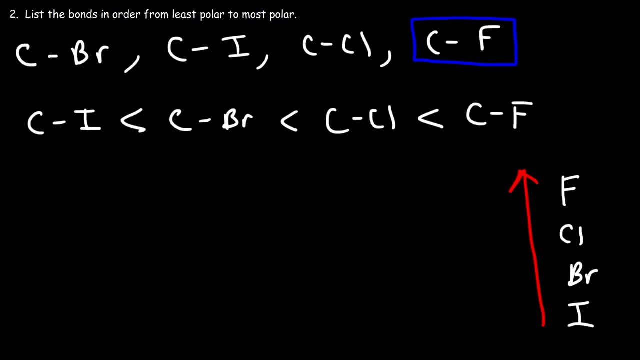 it's easy to rank everything else based on the way it's laid out on the periodic table. Now let's look at the numbers. So keep in mind: carbon is 2.5.. Iodine has an electronegativity value of 2.5.. 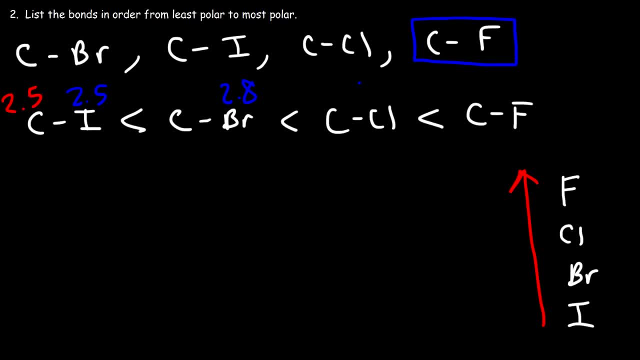 Bromine, it's 2.8.. Chlorine is 3.0.. And for fluorine it's 4.0.. So the EN difference- I'm just going to write the number in green- The EN difference between carbon and iodine is 0.. 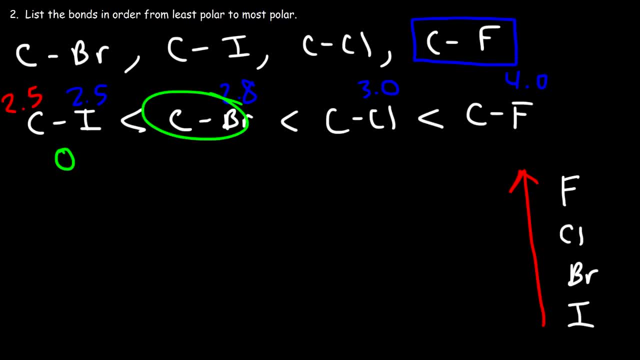 The electronegativity difference between these two elements, that's 2.8 minus 2.5,, so that's 0.3.. And 3 minus 2.5,, that's 0.5.. And 4 minus 2.5 is 1.5.. 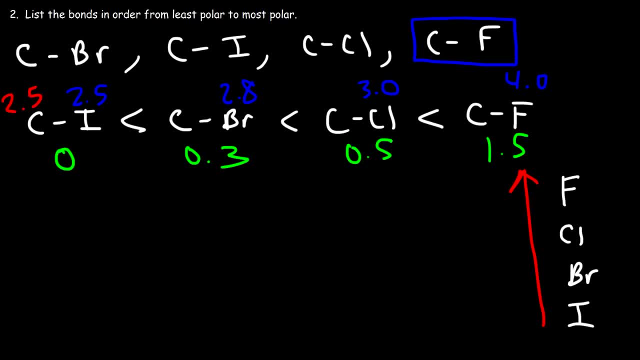 Now keep in mind: in order to have a polar covalent bar, the electronegativity difference has to be 0.4 or less. So therefore these two bonds is relatively nonpolar when you just analyze the electronegativity difference alone. 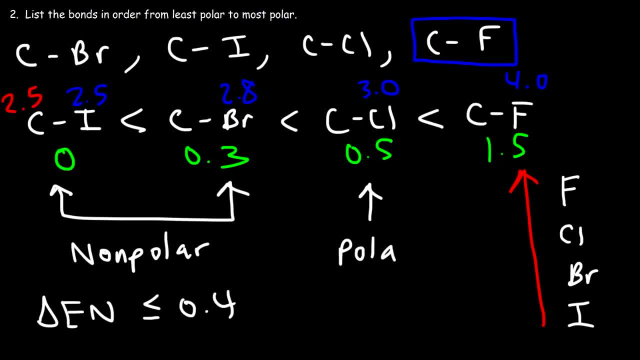 The carbon-chlorine bond is considered to be a polar covalent bond And the carbon-fluorine bond it's highly polar, So it's the most polar bond in this group, Based on the EN difference. Now let's work on one more problem. 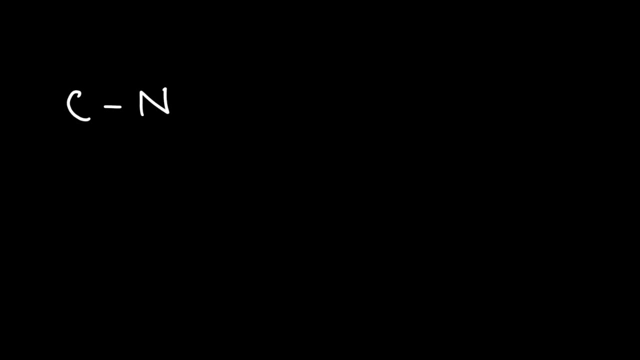 Consider the bonds carbon and nitrogen, carbon and hydrogen, and then carbon and carbon. So in this example I'm going to rank it from most polar to least polar, as opposed to the last example, which was least polar to most polar. So go ahead and try it.